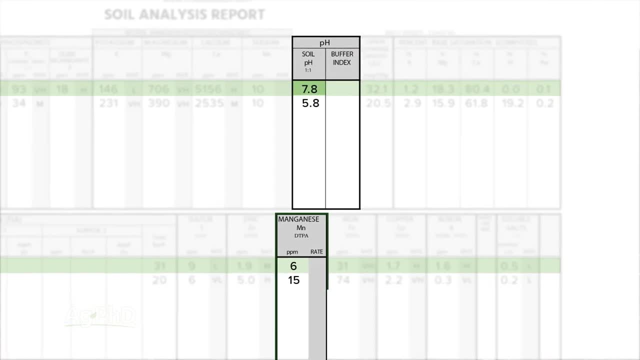 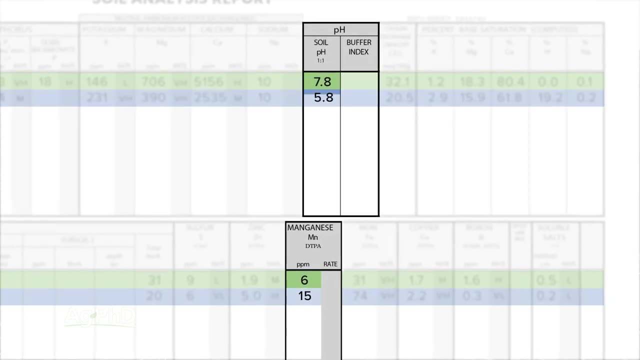 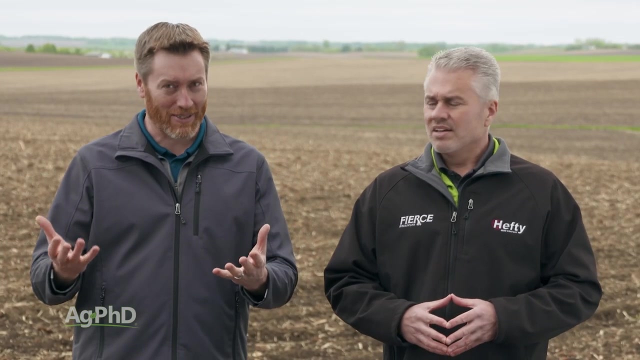 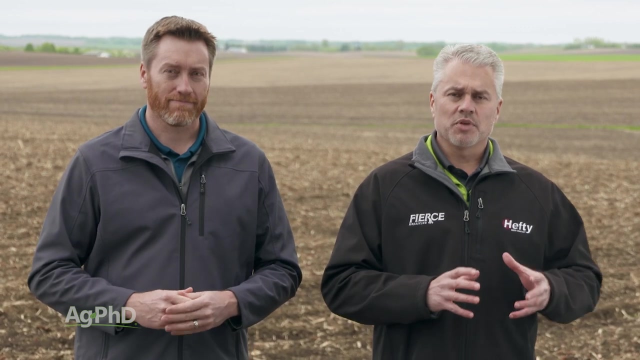 especially, or even some of the upper 6s, we saw lower levels of manganese on many of the tests And when we saw lower soil pHs, like low 6s, upper 5s, we saw higher availability of manganese. Do you see a correlation here with soil pH and potential nutrient tie-up, DARREN? Alright, I want to give you a very specific example with one of the primary nutrients: phosphorus. What happens with phosphorus is it's usually in the phosphate form and in high pH soils. 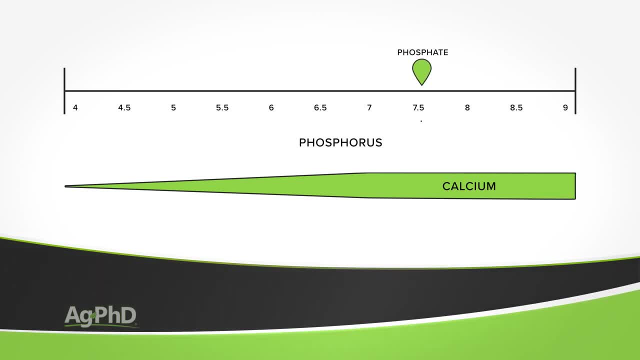 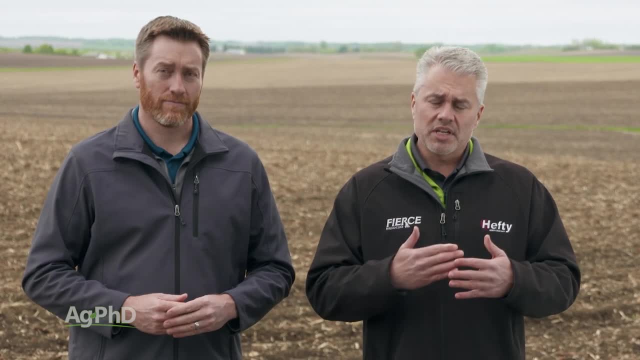 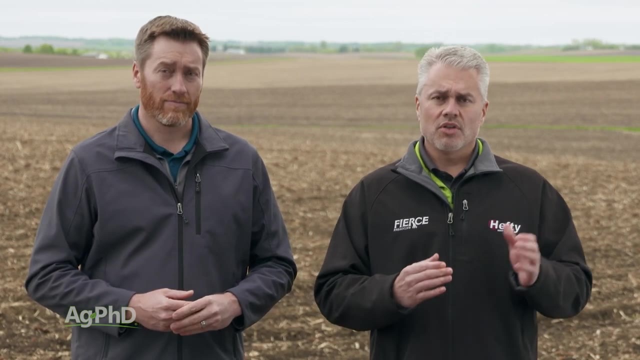 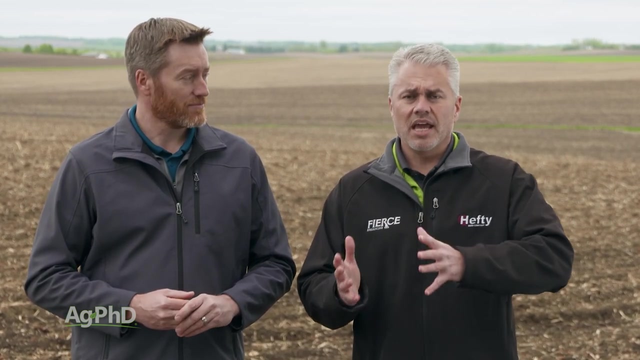 there's typically excess calcium. Well, calcium can bind with phosphate to form calcium phosphate, which unfortunately is insoluble in water. When it doesn't dissolve in water, that means the plant can't bring it in. It's not in a form the plant can use. So it's all because the soil pH gets so high and then we start seeing that excess in calcium and the binding with phosphate. Now the same thing can happen with phosphorus when we get to the lower pHs, and then we start seeing that excess in calcium and the binding with phosphate. Now the same thing can happen with phosphorus when we get to the 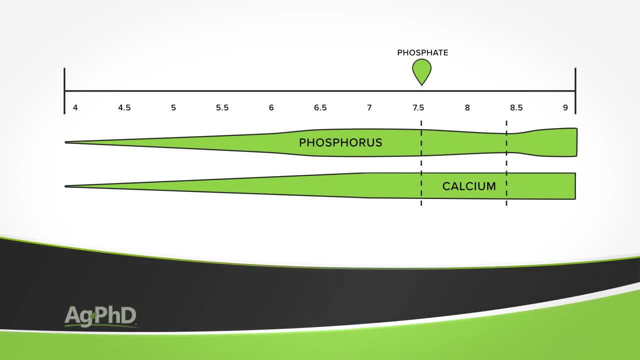 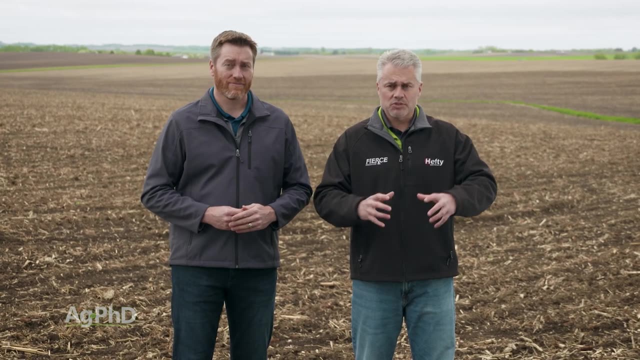 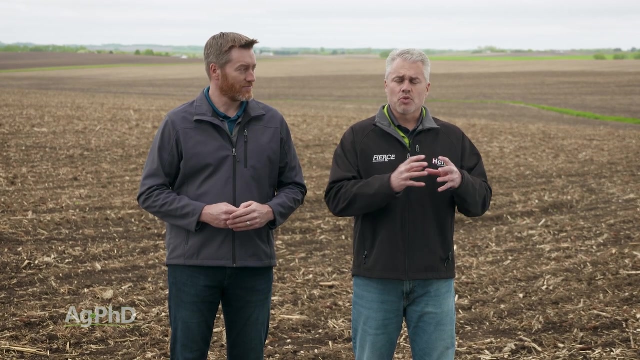 lower pHs. So that calcium thing happens predominantly in the 7.5 to 8.5 range for pH. When the pH is low- let's say it's down in the 5s- we'll commonly see phosphate binding with iron. When the pH is down in the 4s, we commonly see phosphate binding with aluminum. Well, in either case there's phosphorus in the soil but unfortunately it's binding with another nutrient so the plants can't get it and use it. That's a real problem. By simply getting the soil pH in the appropriate range, 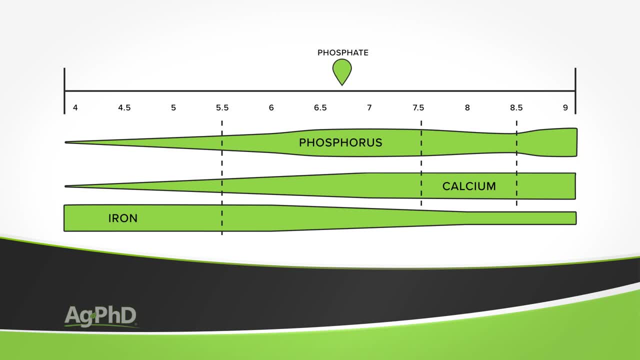 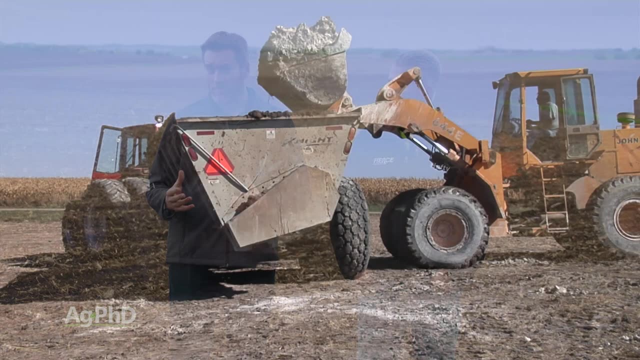 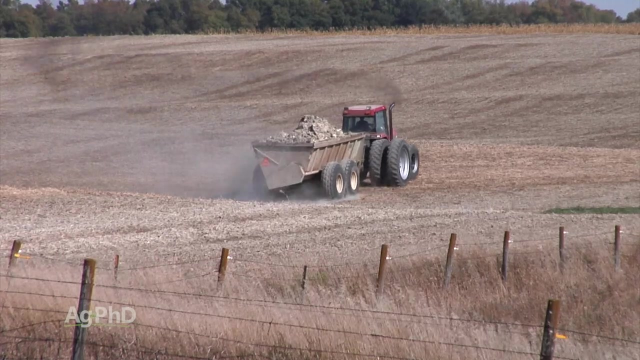 let's say around 6,, 6.5,, 7, somewhere in that range. phosphorus becomes a lot more available than it is when the pH is too low or too high. Now, if your pH is too low, one of the easiest ways to raise that pH up is by applying calcium carbonate. This is something that could be used in your lawn. it could be used in fields, certainly could be used in gardens as well. One spot in particular I'll point out for your lawn is if you have a dog and that dog does his thing.